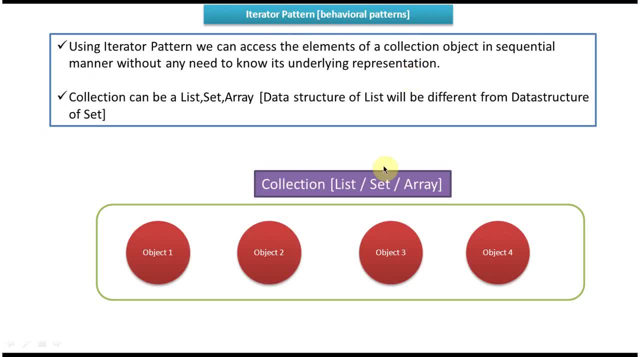 And we will see this diagram, then I will explain. So here you can see collection, Collection, object is nothing but it's a container which contains a lot of objects. So you can see this is the container and it contains four objects: Object 1, object 2, object 3, object 4.. And example of collection is list or set or array. 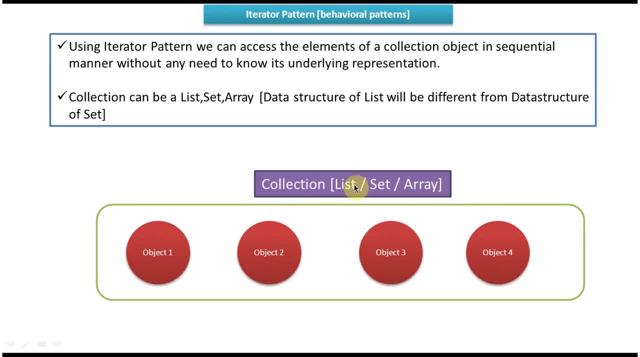 And if you take list, the data structure will be different. And if you take set, data structure of set will be different from the list data structure. And if you take array, array data structure will be different from the set data structure. The storing mechanism of array will be different from set. 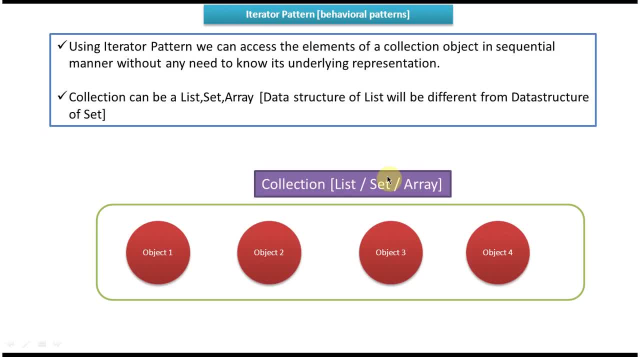 And storing mechanism of list will be different from the set like that. okay, and what is the use of iterator design pattern? is using iterator design pattern, we can access the elements in this container. so suppose we want to get all the objects in this collection in a sequential manner, then we can use iterator design pattern and we can access the objects one. 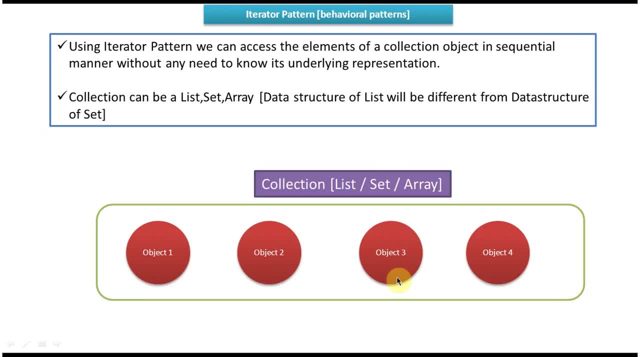 by one and we can process it. so that is the main use of iterator design pattern. okay, and now if you read this explanation, you can understand very clearly. using iterator design pattern, we can access the elements of a collection object. so this is this: object 1, object 2, object 3, object 4 are: 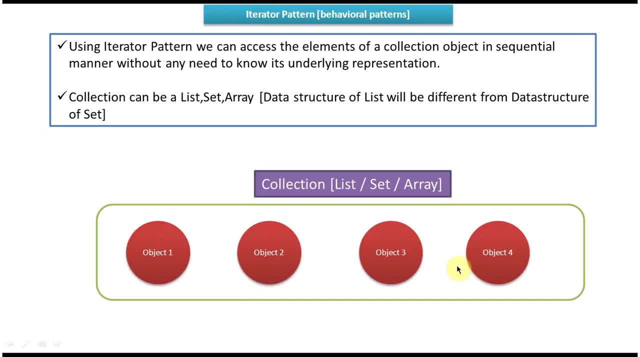 elements of the collection object. using our iterator design pattern, we can access in a sequential manner without any need to know the underlying representation. so we, if you are using iterator design pattern, we no need to worry about internal data structure of list or set or array. okay, we can use iterator design pattern and we can access the elements of a collection object. 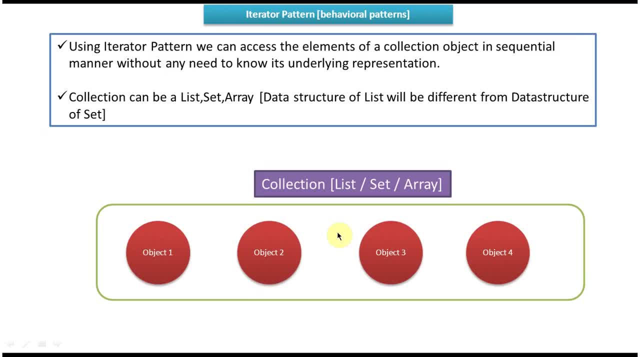 can just use iterator design pattern and access the elements in the collection object. so this is about iterator design pattern and I have created a separate video for how to implement iterator design pattern and I have explained class diagram, all those things. so please log into my channel and 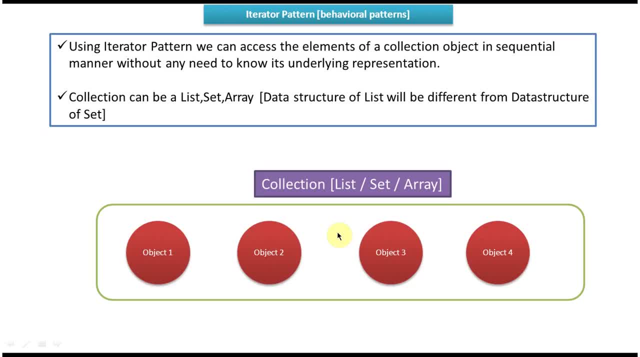 watch that video to understand more about this iterator design pattern. and thanks for watching. bye.